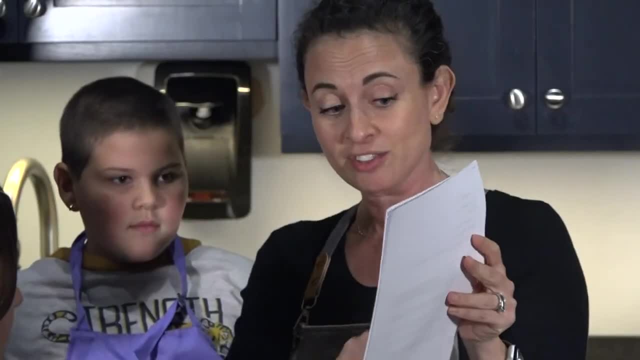 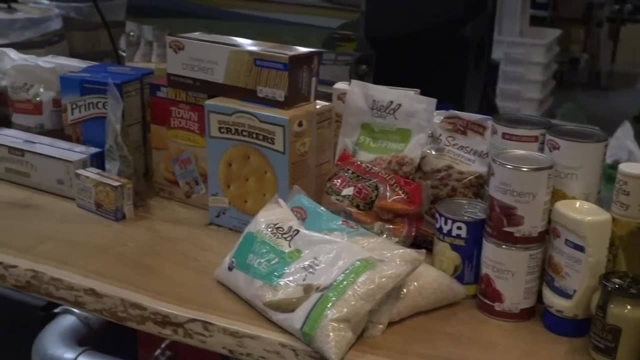 all the pantry items. So here they are. These are the recipes that they're going to be getting: Testing and tasting: Thanksgiving dishes that four families in need will receive ingredients to make at home. You're going to go like this: Okay, You're still starting. 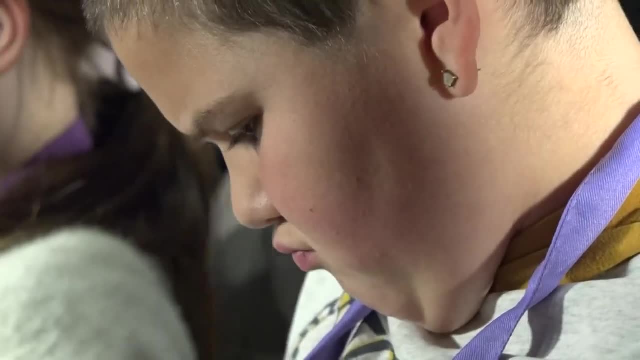 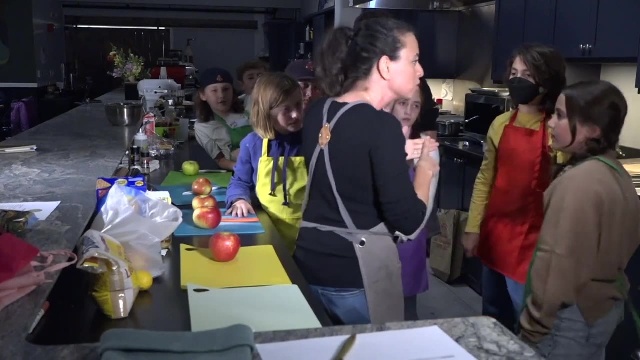 with your point down, Okay, And learning techniques along the way. You can do a small dice, you can do a medium dice, you can do a large dice, you can do a brunoise. Can you guys say that Brunoise? Can you guys all? 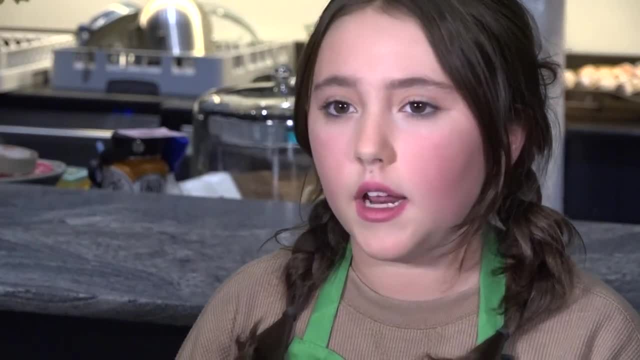 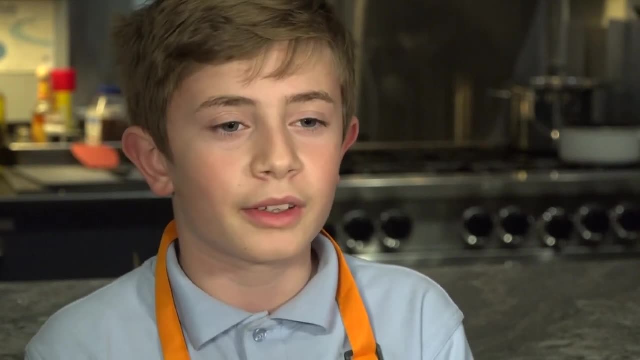 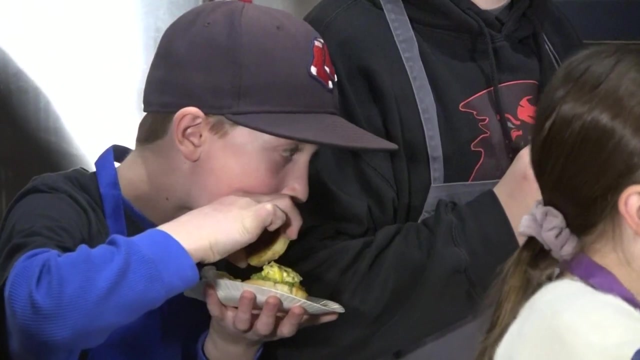 look at me. So we made a pumpkin pie and an apple pie. We learned how to like, cut things safely. We learned how to start the oven, how to bake- I'm always talking about like your taste buds, and how does that work. and 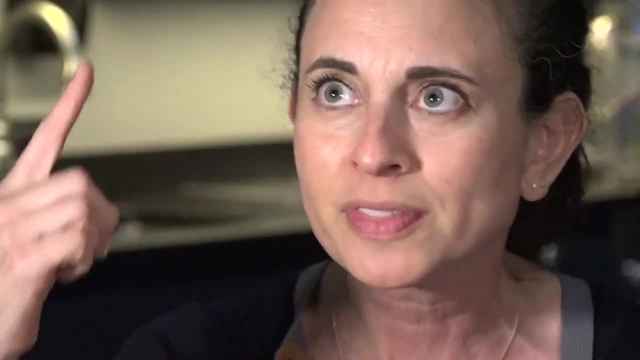 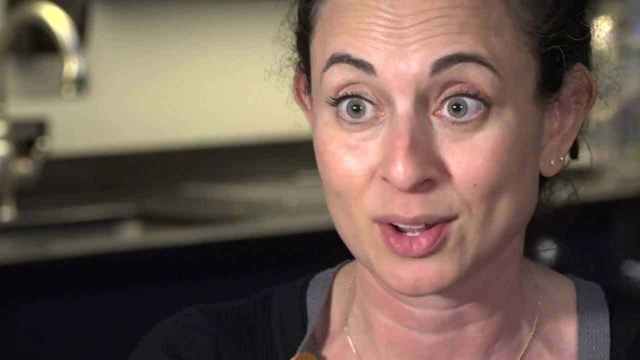 why do you add texture and why would you add seasoning, Like I want them to start thinking now. So one that you're not having kids that are constantly eating macaroni and cheese and you know hot dogs, which we all love, But being able to 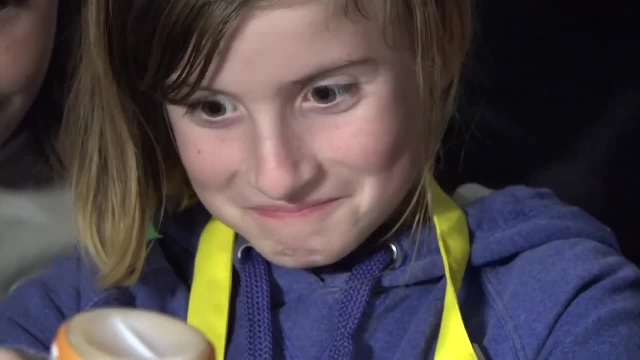 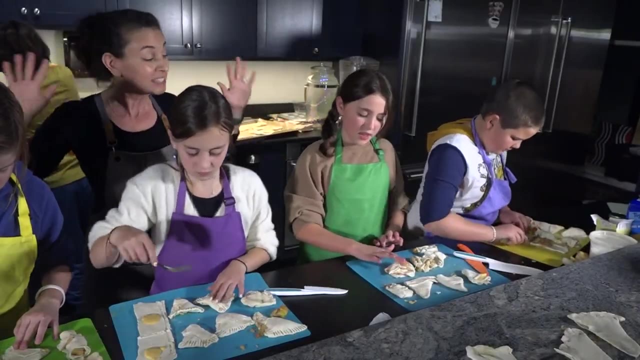 really expand their palate. For Chef Amy, working in the kitchen is not about perfection. It's about having fun And it's your choice. When you're in the kitchen, you can literally do what you want. You know we might fumble and we might. 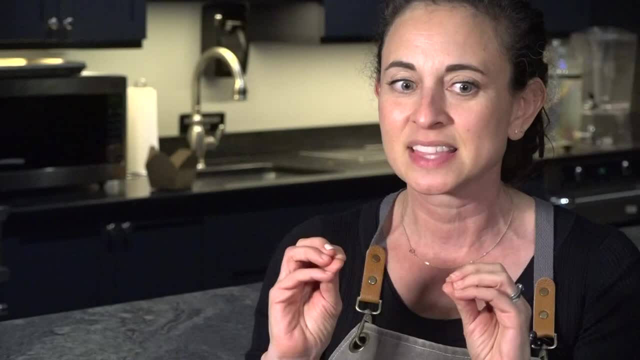 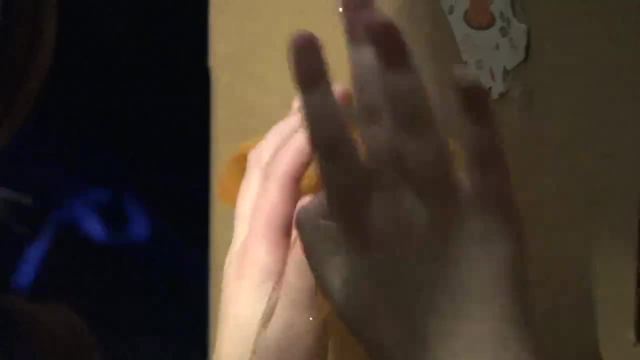 do things here and there and everywhere, But it's like it's the knowledge and the passion behind it which I think is what is so important to teaching the kids. And with that same passion, the kiddos decorated and filled up the boxes with Thanksgiving goods. 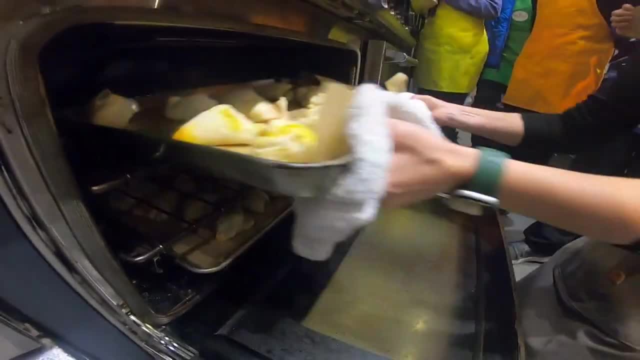 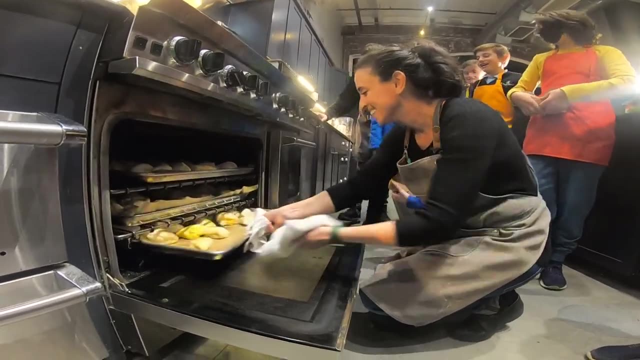 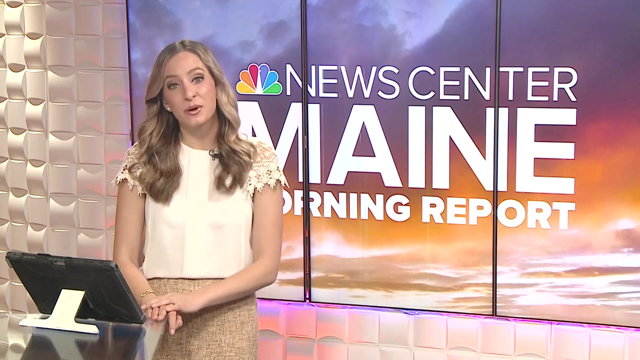 And of course, there is always time to enjoy the treats. Oh my goodness, Oooh Ah Woo. These are great. Chef Amy's classes are done for the season, but registration will soon open for the next season, in March. 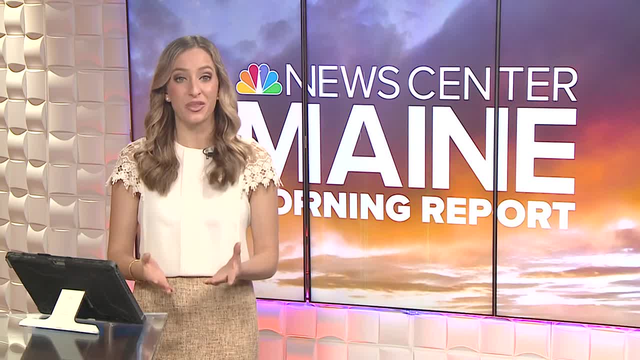 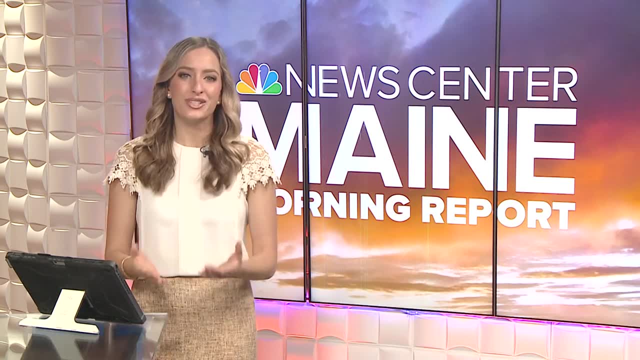 At the end of those classes the kids will prepare a sit down dinner for parents with everything they've learned and the money raised will go to Full Plates- Full Potential to help families in need. If you're interested in Chef Amy's cooking classes for your kiddos at Rhonda Bean in Portland.